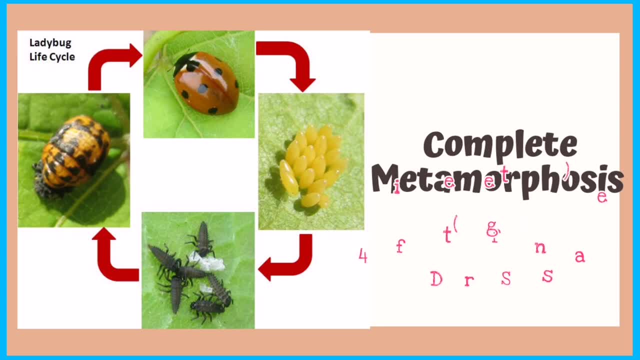 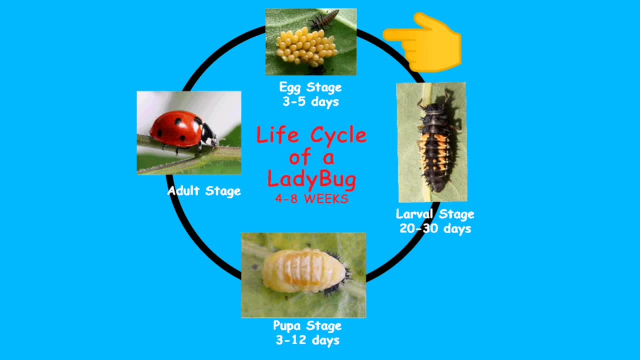 This is an example of metamorphosis. This is an example of metamorphosis. This is an example of complete metamorphosis. This is an example of metamorphosis. This is an example of metamorphosis crisis. The responding metamorphosis is. 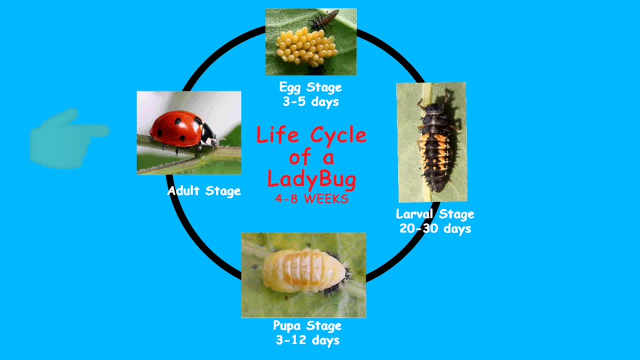 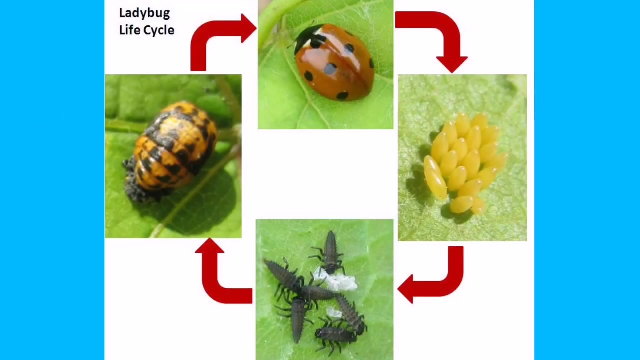 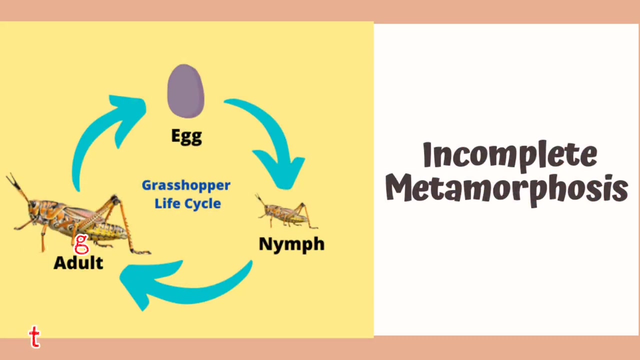 first and finally, the grown adult. the adult ladybug emerges from the pupa. the adult can fly and reproduce, and that commends our life cycle of a ladybug. to recapitulate the four stages, you have to remember the eggs, larva, pupa and adult. number two- incomplete metamorphosis. 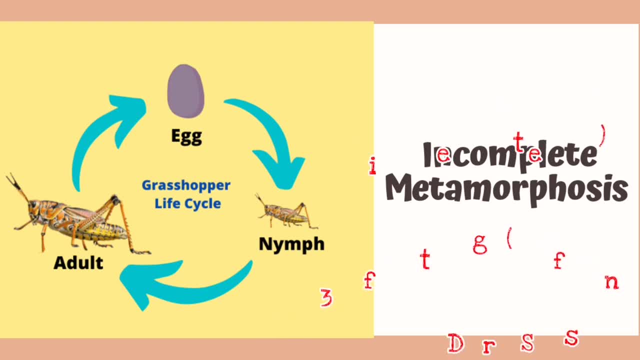 some insects, like dragonflies, grasshoppers and cicadas, go through an incomplete metamorphosis. after hatching, these insects will look like their parents. they will go through changes as they grow, but the way that they look will not change much. why? because the development during an incomplete 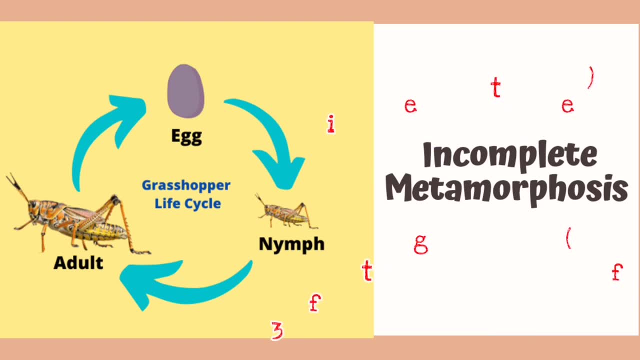 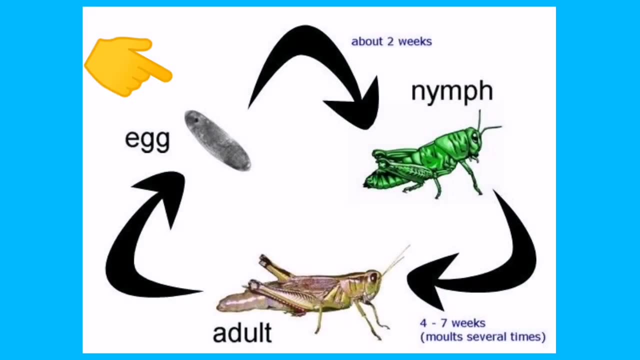 metamorphosis. an animal will go through three different stages in its life cycle. example: the grasshopper. the first stage started with the eggs. an adult grasshopper lays its eggs, then followed by the stage two, which we called nymphs. young grasshoppers, called nymphs, hatch from eggs. they look like adult. 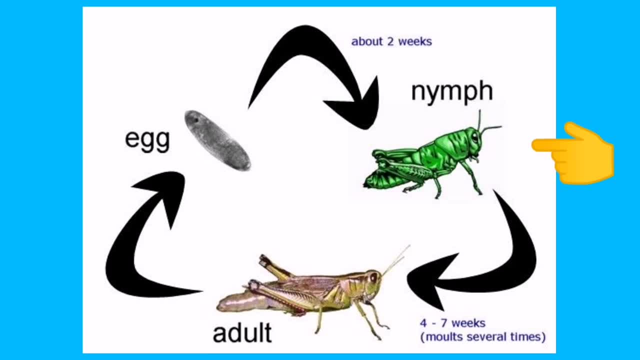 grasshoppers, except they don't have wings yet. as the nymph grows, it sheds its skin several times before it becomes a fully grown adult. each time its wings become bigger, then the nymphs hatch from the eggs. and the nymphs hatch from the nymphs hatch from the eggs. 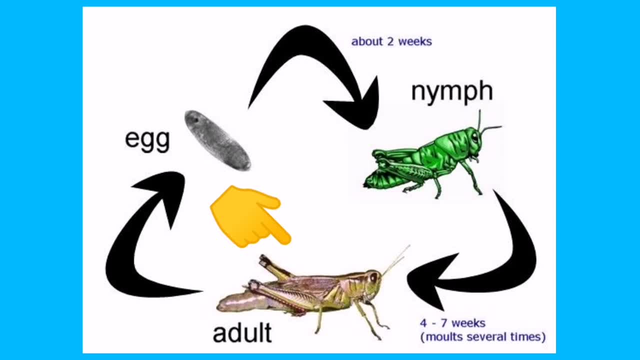 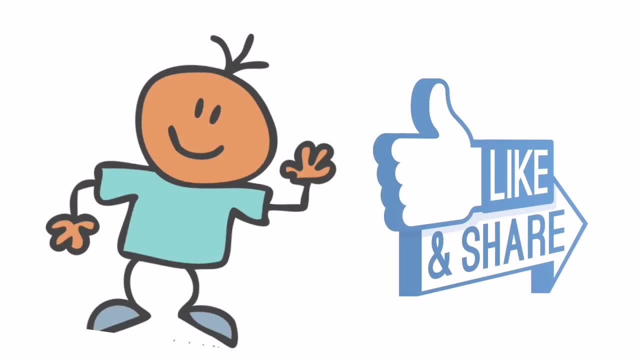 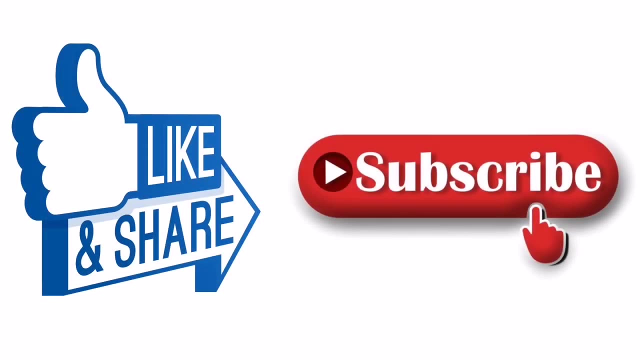 finally, the final shedding produces an adult grasshopper. to recap the three stages, these are egg, nymph and adult. so if you learn new things today, please give a thumbs up and subscribe. please don't forget to hit the bell button to notify you in my upcoming videos. have a great day.